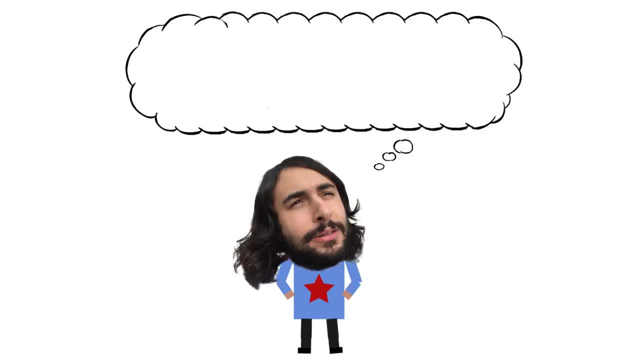 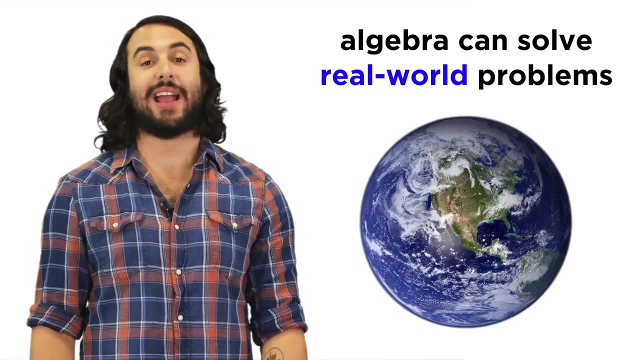 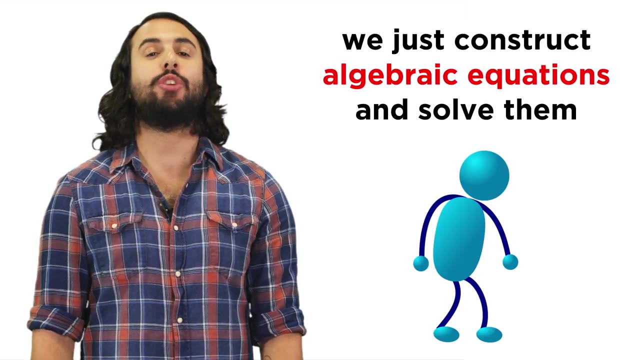 It's Professor Dave. let's look at some word problems. Algebra brings us our first example of how math can be applied in abstract ways to solve real-world problems. A good way to demonstrate this is by constructing algebraic equations that are meant to give. 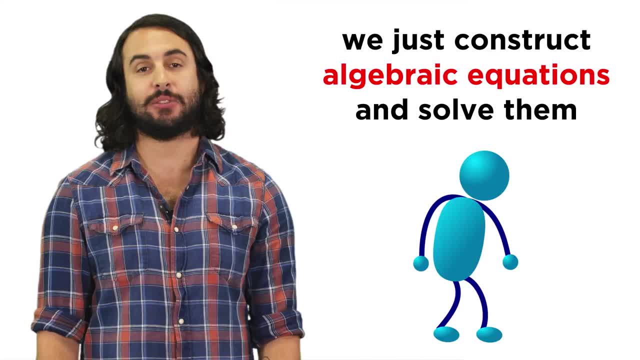 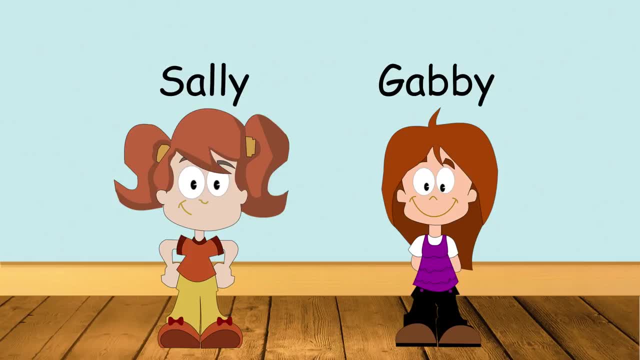 us a solution to a question we might have about a person or any number of things. Take the following example: There are two sisters, Sally and Gabby. Sally is three years younger than twice the age of Gabby. If Gabby is twelve, how old is Sally? 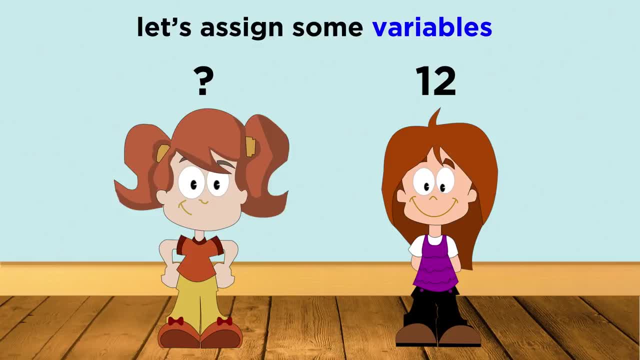 Let's find an equation that can describe this scenario. The first thing we have to do is assign some variables. What do we know and what do we want to know? Well, there's Gabby's age. let's call that G. Then there's Sally's age, let's call that S. 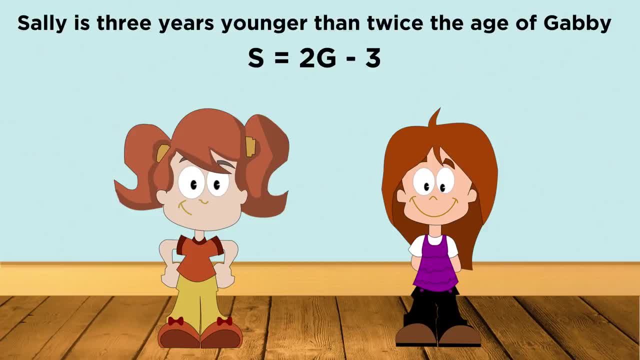 How are these two values related? Well, we know something about S. we know that it is three less than twice G. This means that S equals two G minus three. This equation says exactly the same thing as this sentence, just with symbols instead. 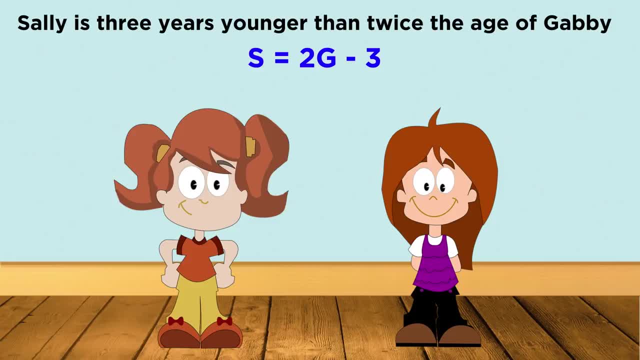 of words. Now we have a very simple equation to solve. We just plug in twelve for G, since that is Gabby's age, double it and subtract three. Sally must be twenty-one. That was an easy one, because we didn't have to do any algebraic manipulation. we just 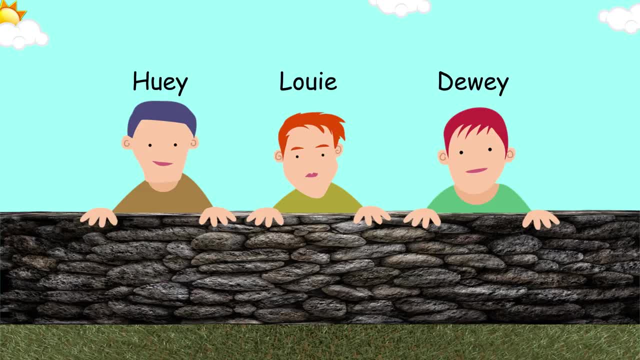 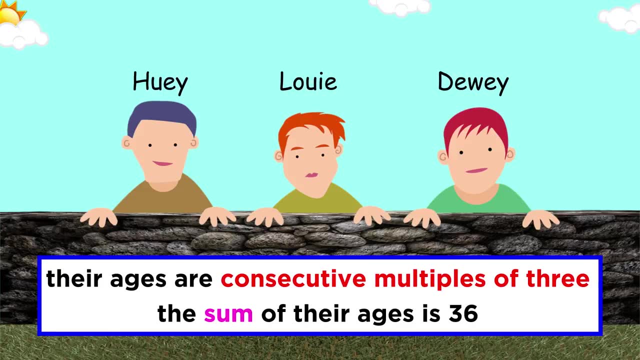 plugged in a number and evaluated. What about something a little harder? Say, there are three brothers: Huey, Louie and Dewey. Their ages are consecutive multiples of three and the sum of their ages is thirty-six. How old are they? 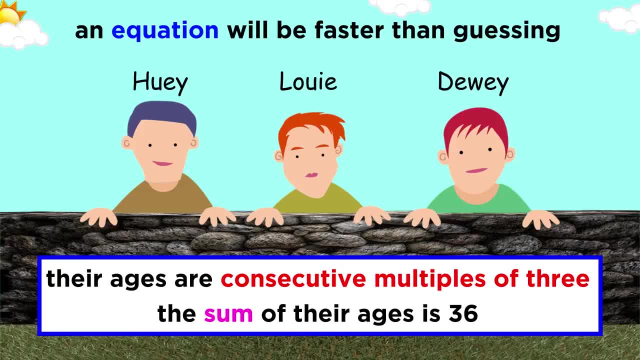 Here we start to see the benefit of constructing an equation, because, while it is certainly possible to just guess and check, Let's look at this equation. Let's look at this equation. When an equation gets sufficiently complex, solving an equation becomes much easier than 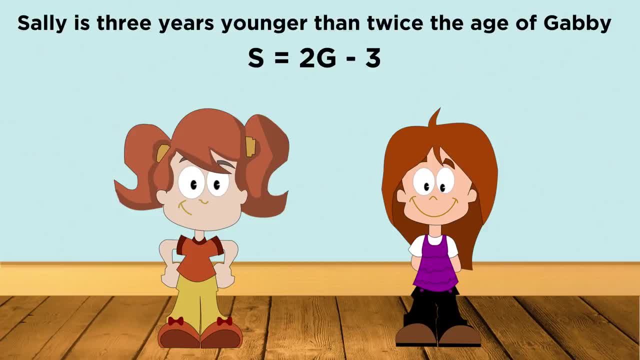 How are these two values related? Well, we know something about S. we know that it is three less than twice G. This means that S equals two G minus three. This equation says exactly the same thing as this sentence, just with symbols instead. 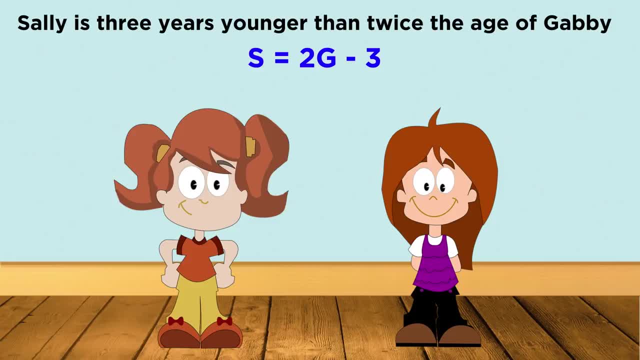 of words. Now we have a very simple equation to solve. We just plug in twelve for G, since that is Gabby's age, double it and subtract three. Sally must be twenty-one. That was an easy one, because we didn't have to do any algebraic manipulation. we just 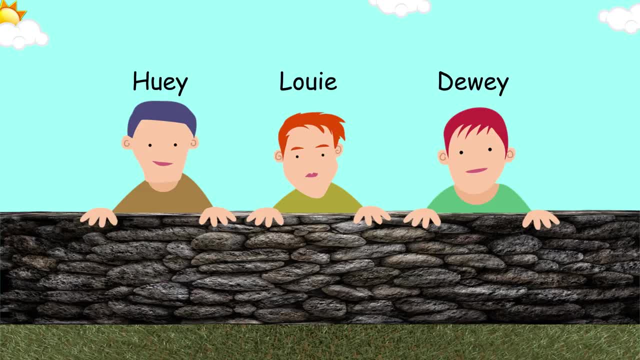 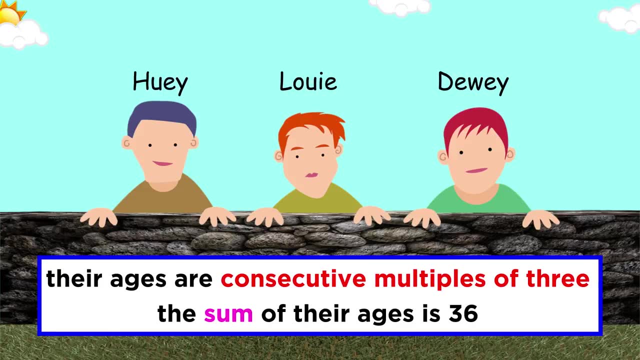 plugged in a number and evaluated. What about something a little harder? Say, there are three brothers: Huey, Louie and Dewey. Their ages are consecutive multiples of three and the sum of their ages is thirty-six. How old are they? 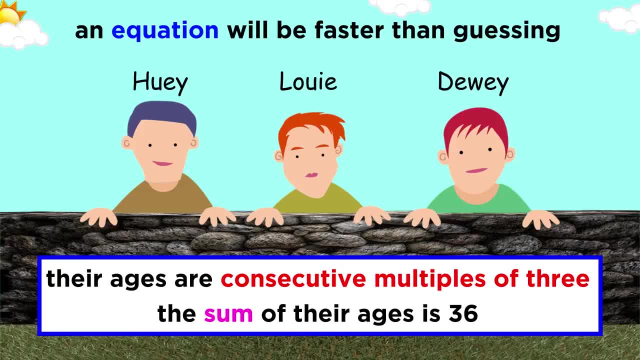 Here we start to see the benefit of constructing an equation, because, while it is certainly possible to just guess and check, Let's look at this equation. Let's look at this equation. When an equation gets sufficiently complex, solving an equation becomes much easier than 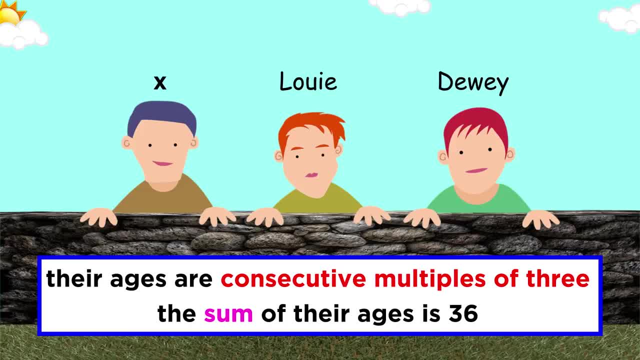 guessing the answer. Let's say the youngest brother has an age equal to X. What would be the other two ages in terms of X? Well, if the ages are consecutive multiples of three and each multiple is three more than the last, then the other two ages must be X plus three and X plus three plus three. 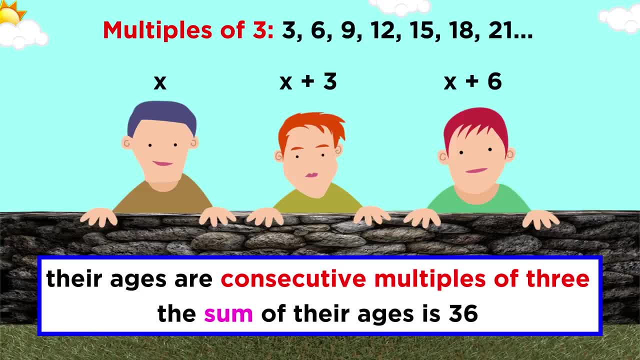 or X plus six. Then it says that the sum is thirty-six. Sum means we add them up. so X plus X plus three plus X plus six equals thirty-six. Now all we have to do is simplify Three X's make three X, and three plus six is nine. 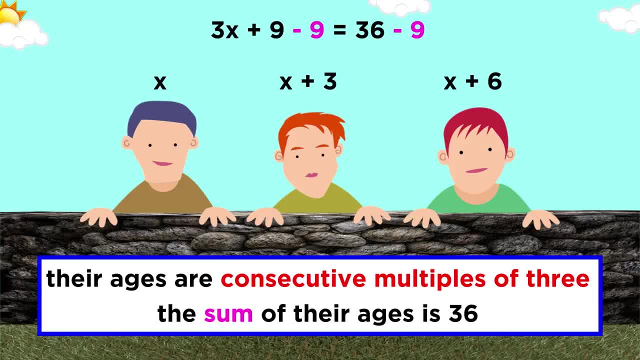 Now we have three. X plus nine equals thirty-six. Subtract nine from both sides to get twenty-seven. divide both sides by three and we get X equals nine. Since X is the age of the youngest, the ages of the brothers are nine, twelve and fifteen. 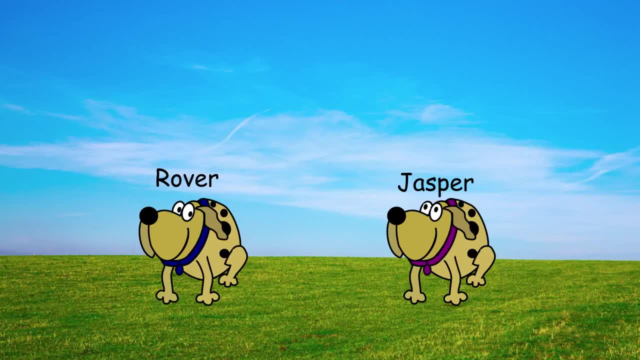 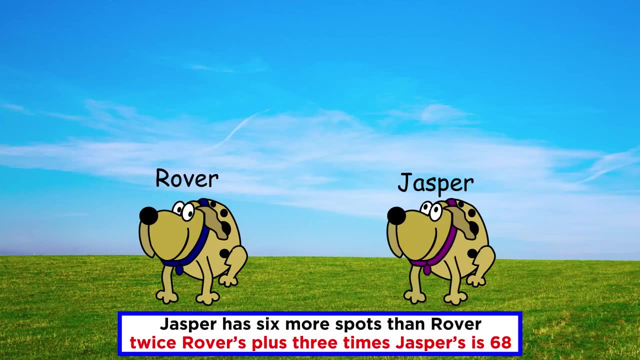 Let's try one more. Rover and Jasper are dogs and they each have spots. Jasper has six more spots than Rover does, and twice the number of Rover's spots plus three times the number of Jasper's spots equals sixty-eight. How many spots do they have? 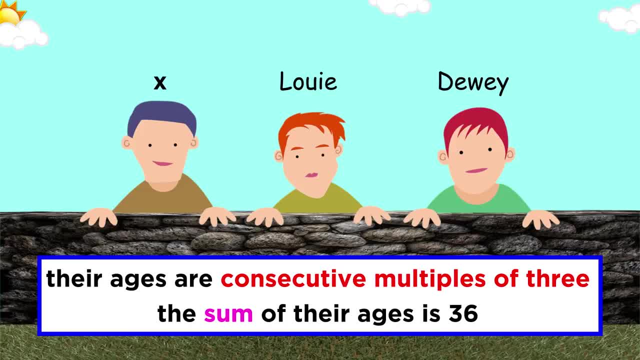 guessing the answer. Let's say the youngest brother has an age equal to X. What would be the other two ages in terms of X? Well, if the ages are consecutive multiples of three and each multiple is three more than the last, then the other two ages must be X plus three and X plus three plus three. 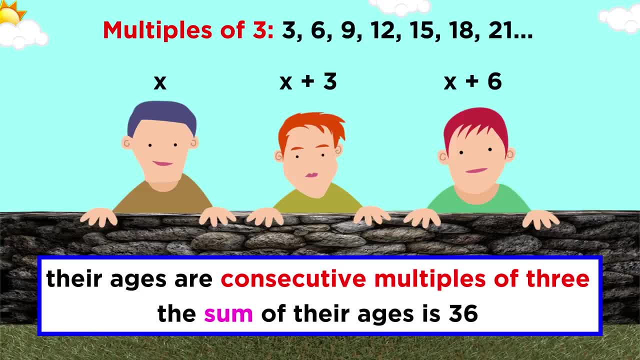 or X plus six. Then it says that the sum is thirty-six. Sum means we add them up. so X plus X plus three plus X plus six equals thirty-six. Now all we have to do is simplify Three X's make three X, and three plus six is nine. 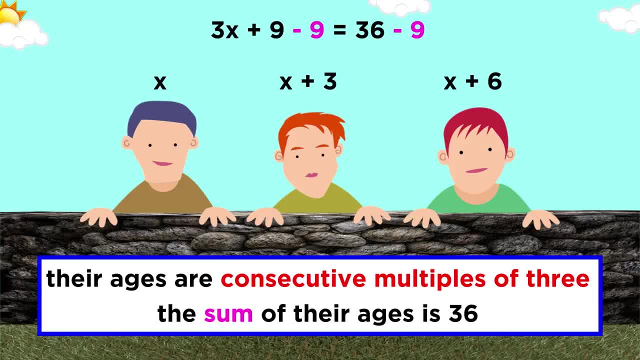 Now we have three. X plus nine equals thirty-six. Subtract nine from both sides to get twenty-seven. divide both sides by three and we get X equals nine. Since X is the age of the youngest, the ages of the brothers are nine, twelve and fifteen. 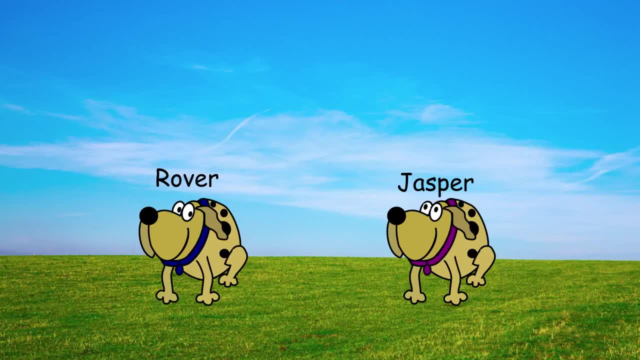 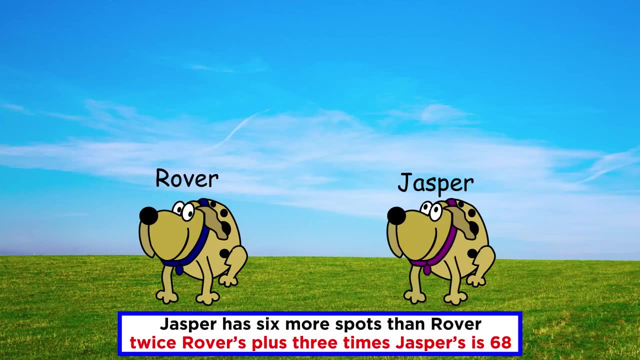 Let's try one more. Rover and Jasper are dogs and they each have spots. Jasper has six more spots than Rover does, and twice the number of Rover's spots plus three times the number of Jasper's spots equals sixty-eight. How many spots do they have? 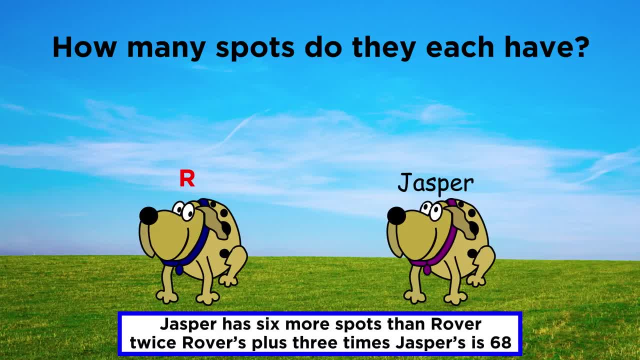 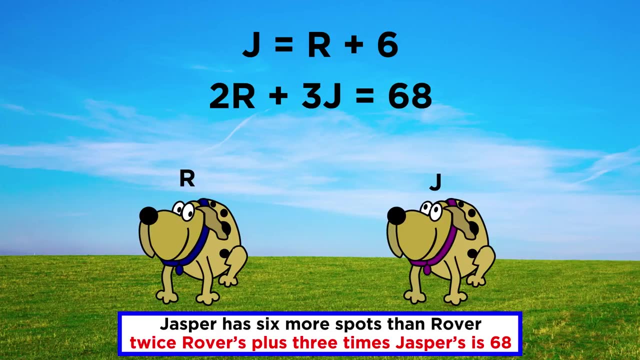 Well, first let's assign the variables. Rover's spots are represented by R and Jasper's by J. How do these variables relate to one another? Well, if Jasper has six more spots than Rover, then J equals R plus six. Then we have this other bit of information whereby two R plus three J equals sixty-eight. 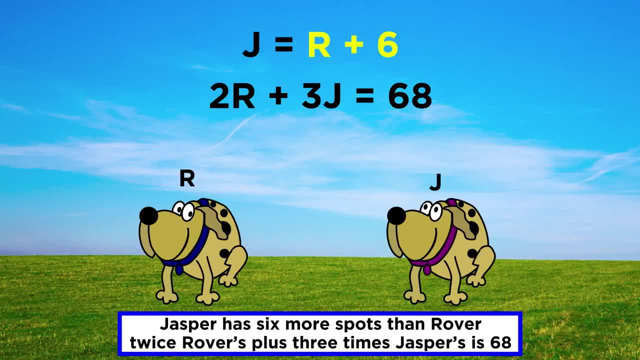 What can we do from here? Well, if J equals R plus six, we can put R plus six in this other equation instead of J, because they are equivalent, This term has to go inside parentheses and we can immediately distribute this: three, That gives us two, R plus three, R plus eighteen. 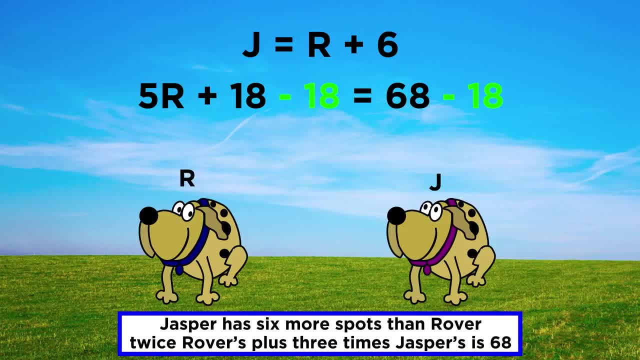 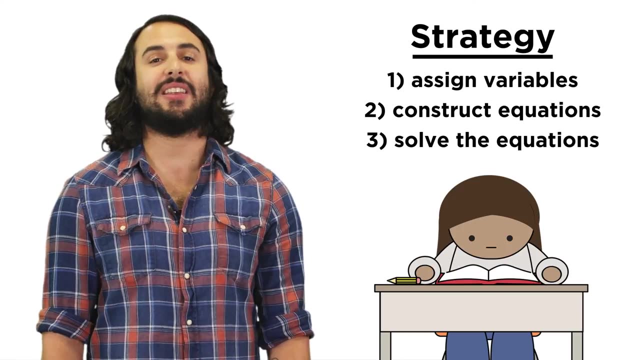 We can combine the R's to get five, R, subtract eighteen from both sides to get fifty, and then divide everything by five to get R equals ten. If R is ten, then J is sixteen and that's all the spots. So we can see that in these scenarios we just have to decide on some variables and 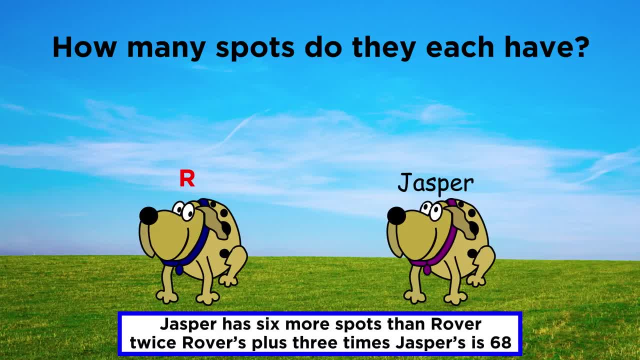 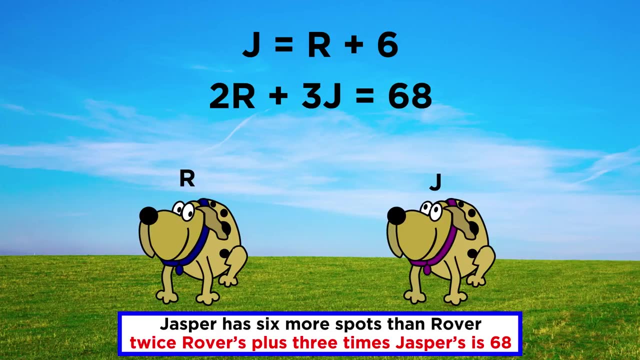 Well, first let's assign the variables. Rover's spots are represented by R and Jasper's by J. How do these variables relate to one another? Well, if Jasper has six more spots than Rover, then J equals R plus six. Then we have this other bit of information whereby two R plus three J equals sixty-eight. 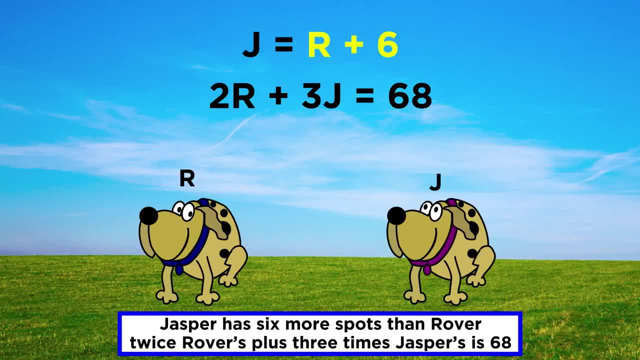 What can we do from here? Well, if J equals R plus six, we can put R plus six in this other equation instead of J, because they are equivalent, This term has to go inside parentheses and we can immediately distribute this: three, That gives us two, R plus three, R plus eighteen. 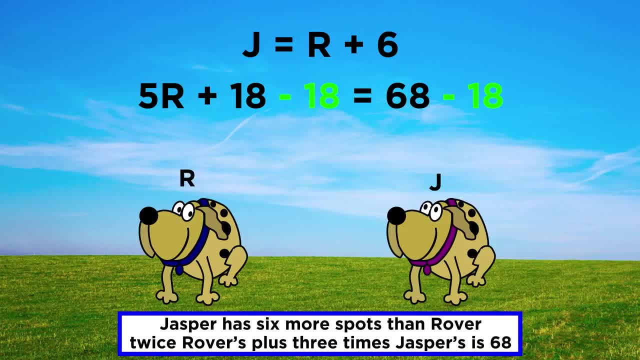 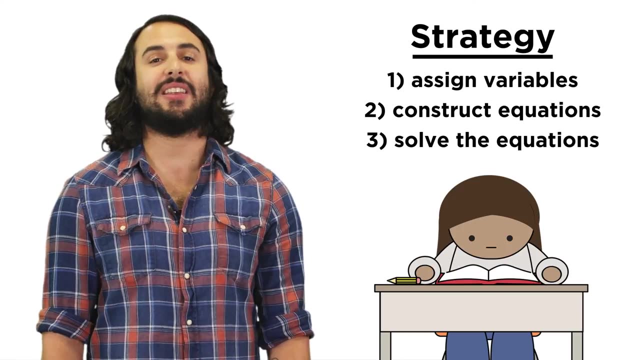 We can combine the R's to get five, R, subtract eighteen from both sides to get fifty, and then divide everything by five to get R equals ten. If R is ten, then J is sixteen and that's all the spots. So we can see that in these scenarios we just have to decide on some variables and 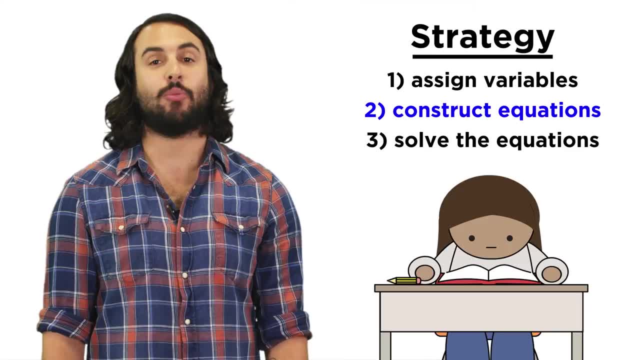 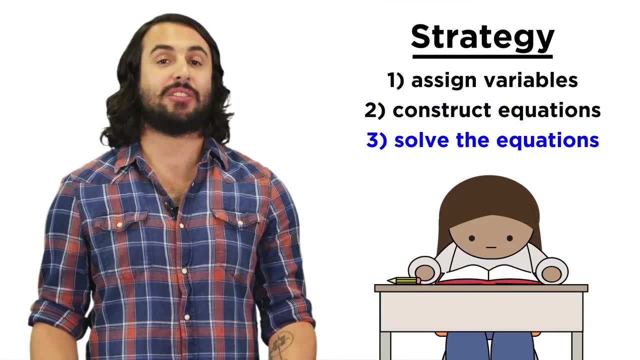 construct whatever equations we can from the information we have. That's the trickier part, because it requires some abstract thought. So let's try this again Once we've done that. solving them is the easy part, as that will be the same old math. 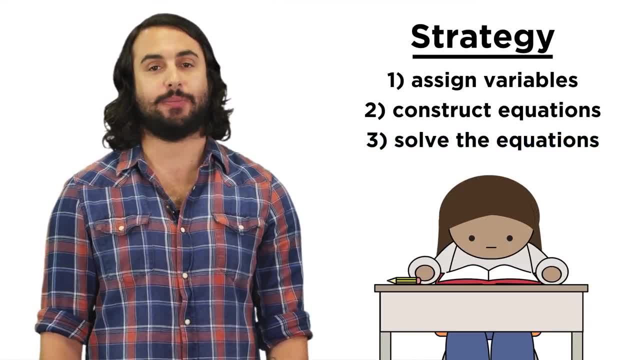 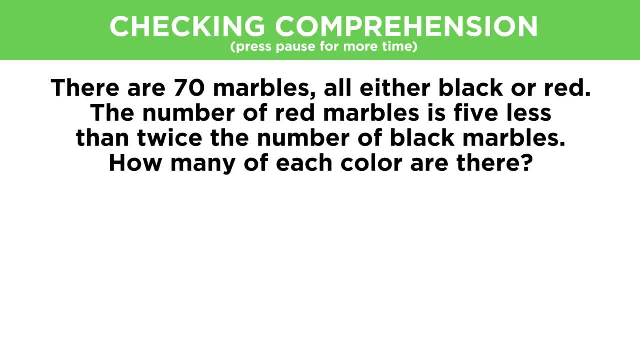 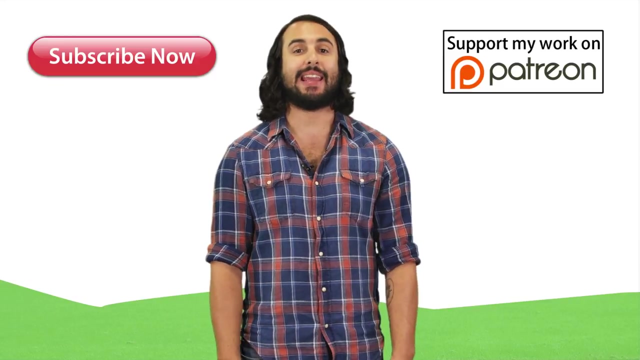 every time. I think you've got the hang of it, so let's check comprehension. I think you've got the hang of it, so let's check comprehension. Thanks for watching, guys. Subscribe to my channel for more tutorials. Support me on Patreon so I can keep making content. 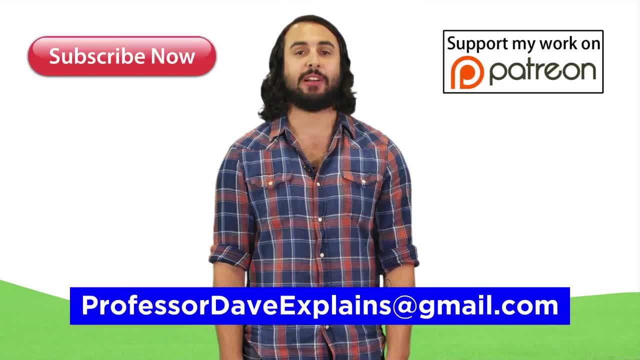 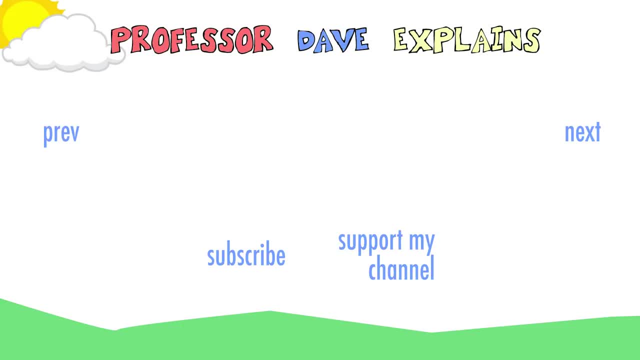 And, as always, feel free to email me professordaveexplains at gmail dot com. I'll see you next time. Bye-bye, Bye-bye.